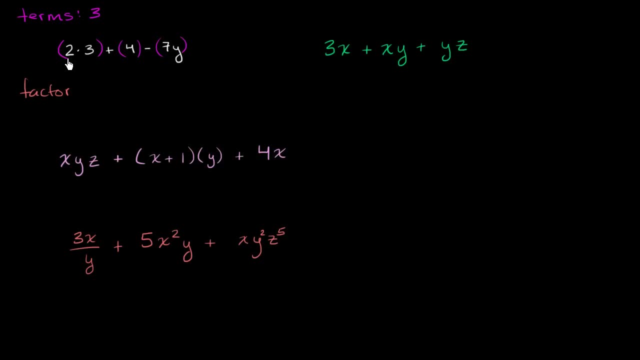 So, for example, if you said: what are the factors of the first term? The first term refers to this one, This one right over here, two times three And there's two factors. There's a two and a three And they are being multiplied by each other. 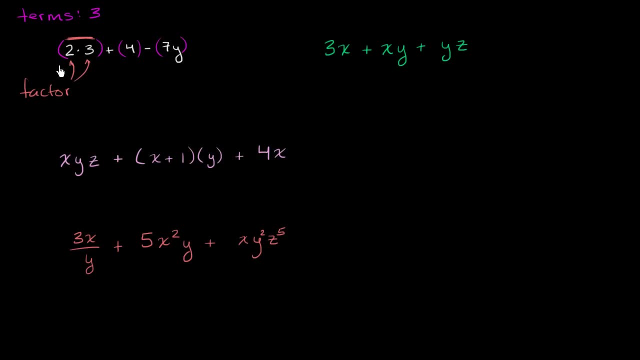 So here you have two factors in the first term. What about the second term? The second term right over here, the second? this was the first term. the second term here has only one factor, Just the four. It's not being multiplied by anything. 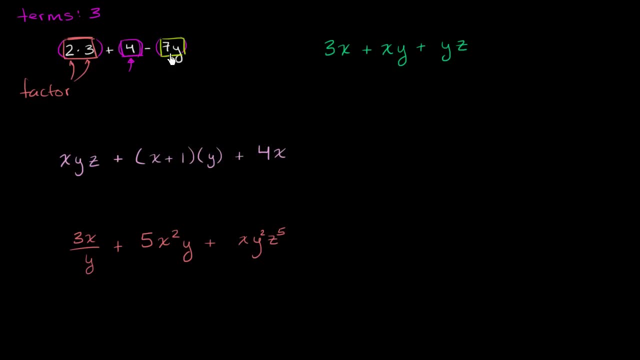 And the third term here once again has two factors. It's the product of seven times y. So we have two factors here. We have a seven and a y. And this constant factor here, this number seven, that is multiplying the variable, also has a special name. 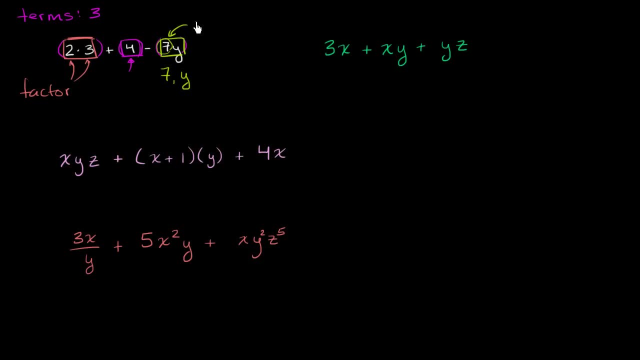 It is called the coefficient of this term Coefficient. And the coefficient is the non-variable that multiplies the rest of the term. That's one way of thinking about it. So here's seven y, Even if it was seven xy or seven xyz or seven xyz squared, that non-variable that's multiplying everything else we would consider to be the coefficient. 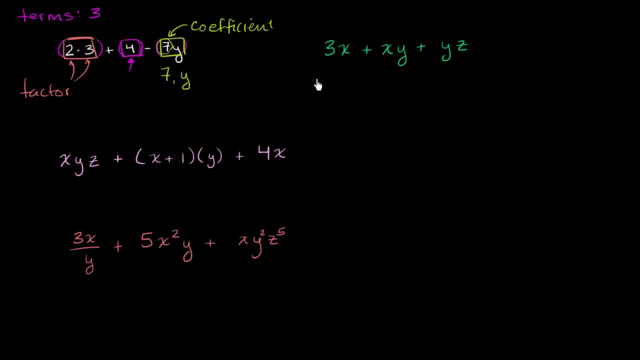 Now let's do a few more examples, And in each of these I encourage you actually right now to pause the video. Think about what the terms are, How many terms are there in each expression, How many factors in each term, And what are the coefficients. 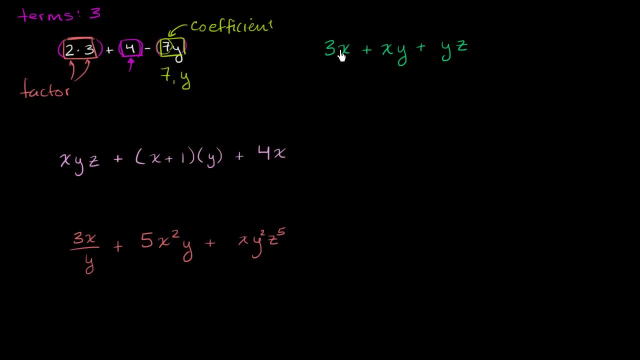 So let's look at this first one. It's clear that we have three things being added together. This is the first term, This is the second term And this is the third term. So this is the first term, This is the second term. 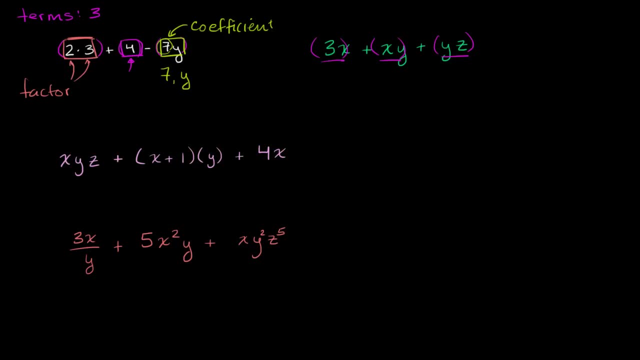 This is the third term And they each have two factors. This first one has the factors three and x, The second one here has the factors x and y, And this third one has the factors y and z. Now, what are the coefficients here? 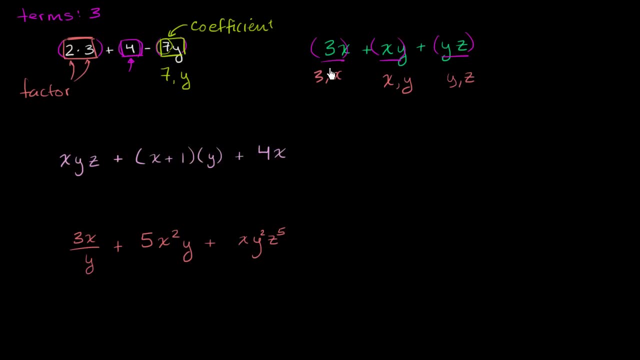 Well, remember, coefficients is a non-variable multiplying a bunch of other variables. And so here the coefficient in this first term right over here, is a three. Now you might be saying, well, what about the coefficients on these terms right over here? 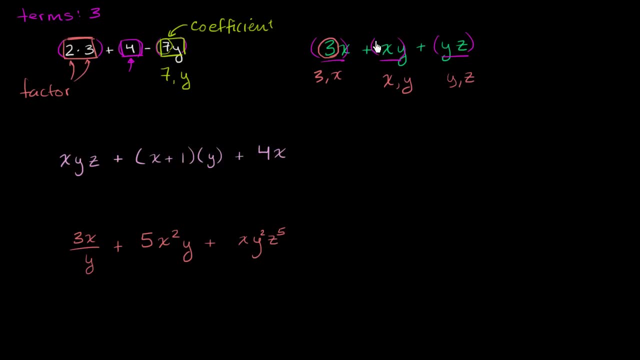 Depending on how you think about it. one way to say is: well, xy is the same thing as one times xy. So some people would say that, hey, you have a coefficient of one here on the xy, Or it's implicitly there. 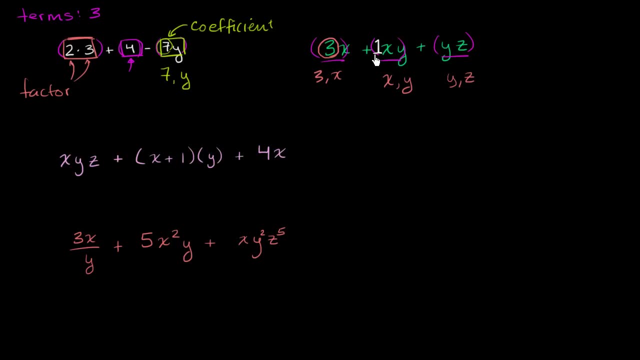 It wasn't written, but you're multiplying everything by one And that might be subject to a little bit of interpretation one way or another. Now, this one is really interesting Because if we look at the bigger expression, if we look at the whole thing, 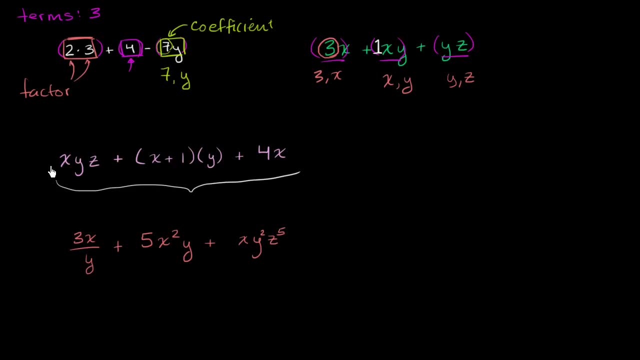 if we look at the whole thing, it's clearly made up of three terms. The first term is xyz, The second term is x plus one, that thing, whole thing times y. And then the third term is 4x. And if you look at that level, if you look at the first term, 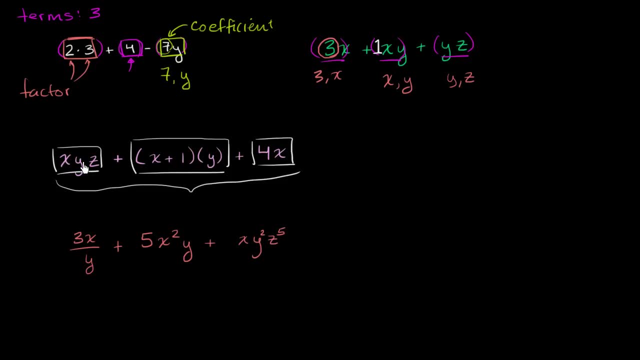 and you say: well, how many factors does that have? Well, you would say that it has three factors: x, y and z. How many factors does the second term have? Well, you could say: well, it has two factors. One factor is x plus y. 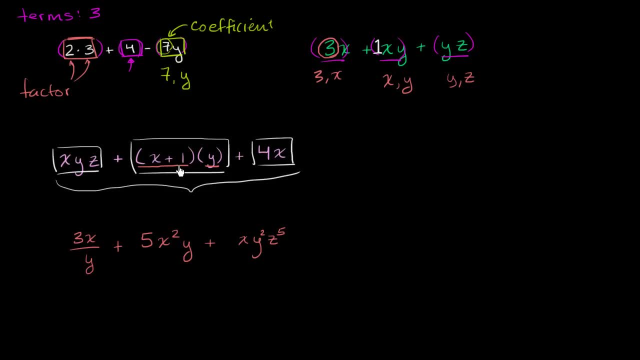 It's multiplying x plus, or sorry, the first factor is x plus one And the second one is y. It's multiplying this expression. This expression itself, this smaller expression itself is one of the factors, And the other one is y. 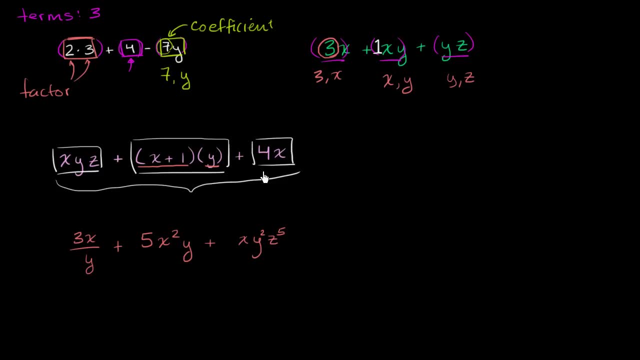 And then this third one also has two factors, A four and an x. And if someone said, hey, what's the coefficient on this term, You'd say, hey, look the coefficient. the coefficient is the four. Now let's look at this one over here. 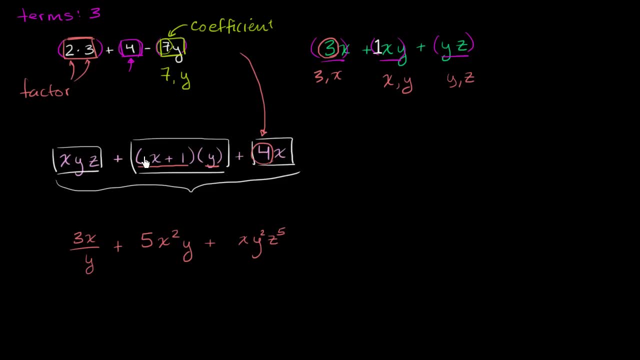 Actually, before I look at that one, what was interesting about this is that here you had a little smaller expression, itself acting as one of the factors. So then you can go and then zoom in on this expression right over here and you can ask the same question. 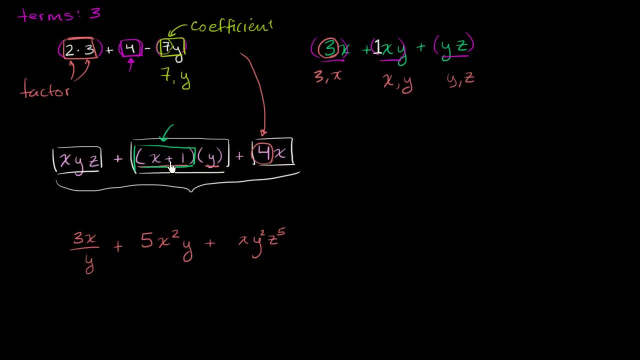 On this smaller expression. how many terms does it have? Well, it has two terms: An x and a one. Those are the two things being added or subtracted And each of them have exactly one factor. So when we're giving these, you can keep nesting these expressions. 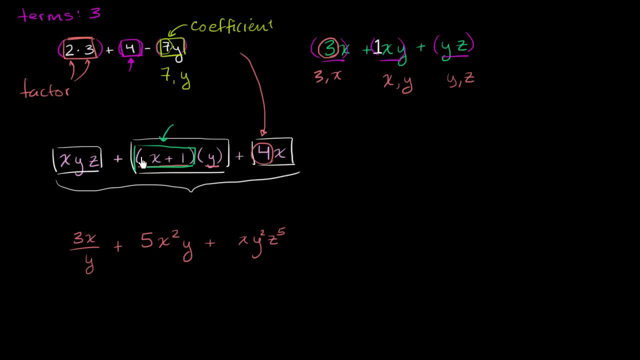 to think about. when you talk about terms or factors or factors of terms, you have to really specify what part of the nesting you're thinking about. If you're talking about the terms of this whole expression, there's one, two, three. 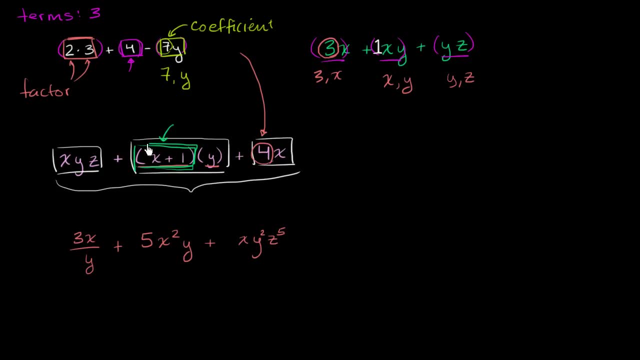 But then, if you go, you can look at this sub-expression, which itself is a factor of a term, and say: oh well, there's only two terms in this one. Now let's look at this one. How many terms? Well, once again, there's clearly three.